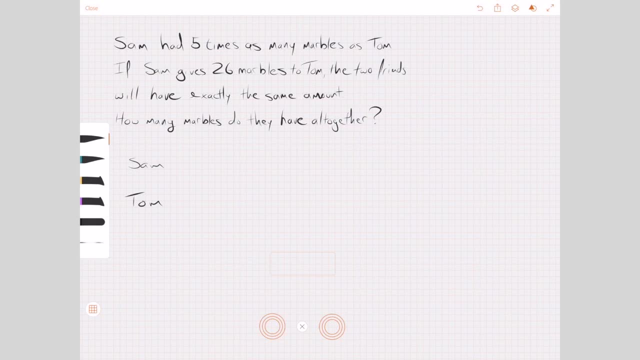 represent that in our problem simply by drawing a series of bars. So if I use this here to represent the quantity that Tom has Like this Right, Then for Sam what I need to do is I need to draw five of these bars at the same size, because he has five times as many. So hopefully all of you will see. 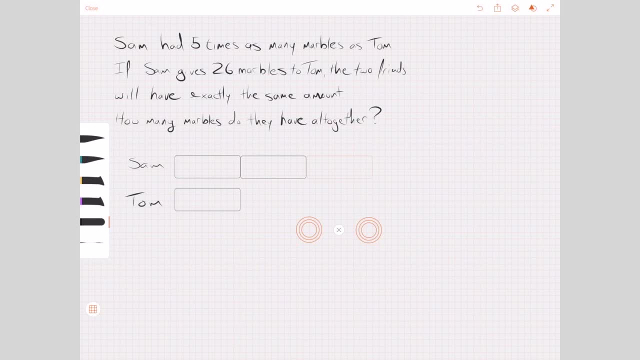 that. that's quite an easy way to visualize the problem. So this is a before and after problem. So this is the before situation. So Sam starts off with five times as many as Tom. Now the other thing that we know in our problem is is that 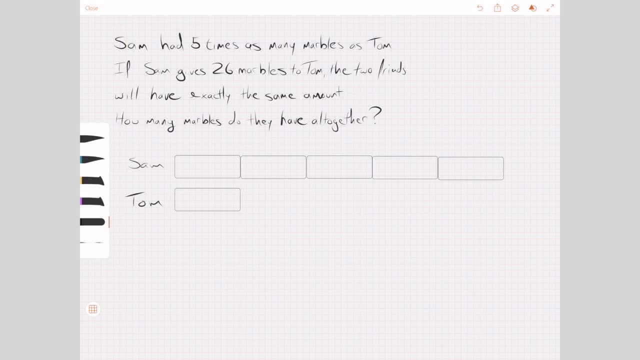 um, the two boys, uh, end up with the same amount, Right? Um, and that Sam gives 26 marbles to Tom. So let's go and color these up, because I think I have a feeling that this is going to help us out. So I'm going to color Sam's over here in yellow. See if I can get this. 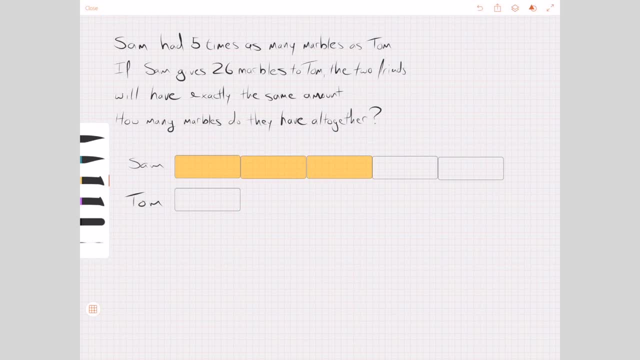 to work. Yeah, there we go. So these are Sam's right, And they're all yellow, Okay, And he's got five times as many as Tom, which I'm going to color in this pink color here. This is our current situation. Now something happens. 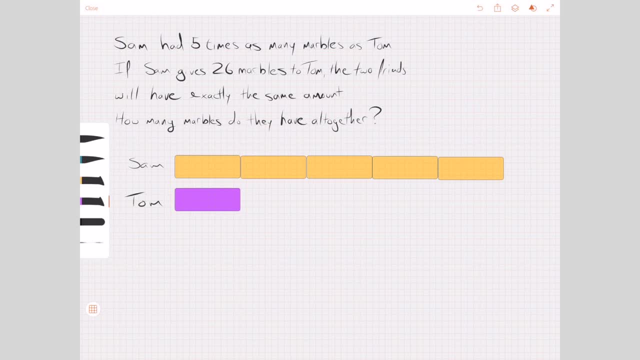 Sam gives some of his marbles to Tom and- uh, we know how many- 26.. And when he does that, both of them will end up with the same amount. Now, if we look here, we can see quite clearly that if Sam- and this is where the aha moment is for most pupils is when they 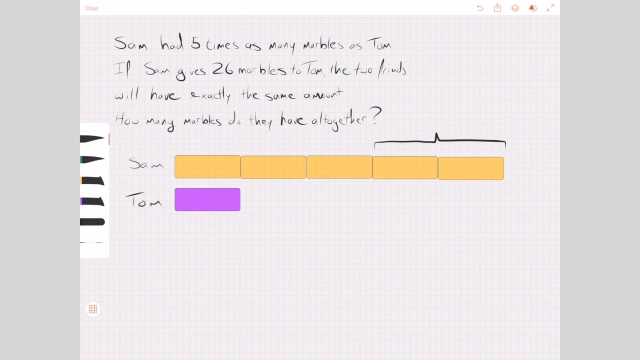 recognize that if Sam gives these two bars here to Tom, right, they will end up with the same amount. So if I just go back here and draw, and I'm going to color this one in yellow and I'm going to draw two more bars over here for Tom, So these are going. 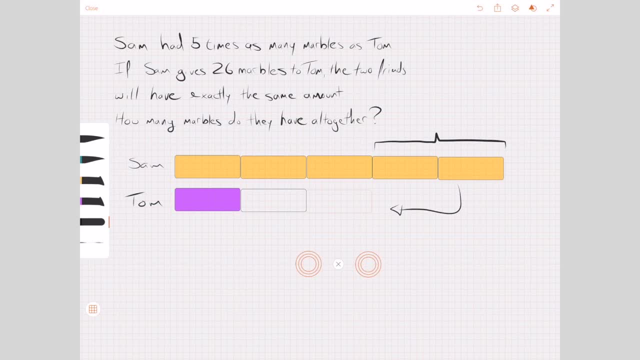 to be: um, these are going to be quantities of marbles that Tom receives from Sam. right, There's two right And we can hopefully what we can recognize is there's a before and after situation. So I'm going to draw a line here right to to show the two. So 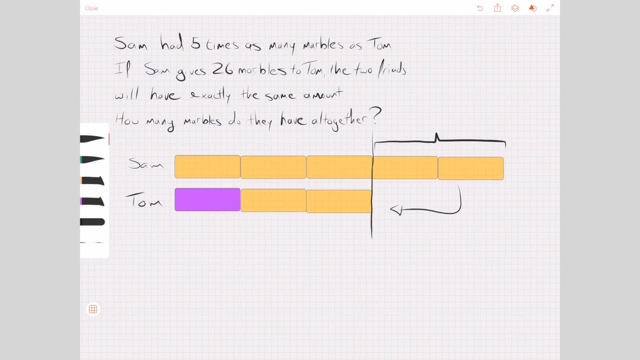 when Sam gives two of his over here to Tom, they will end up with the same amount. So this is the same amount, right? I hope that makes sense. Now what's the other thing that we know? We know how many Sam gave to Tom, right? So Sam gave 26 marbles to Tom. 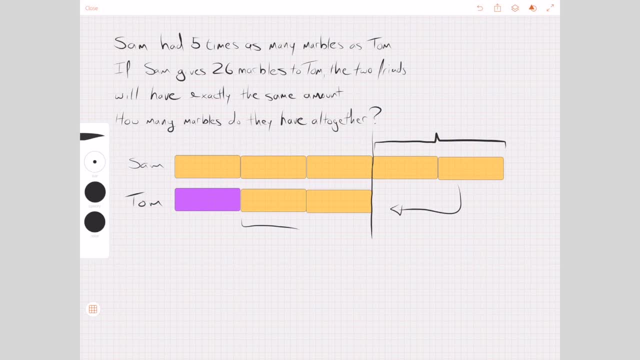 So this amount of marbles here right is 26.. Okay, So we haven't even looked at the question yet, We've just looked at the facts that we've been given. So you see, at this point here I hope that most children will recognize that if they know that they're going, 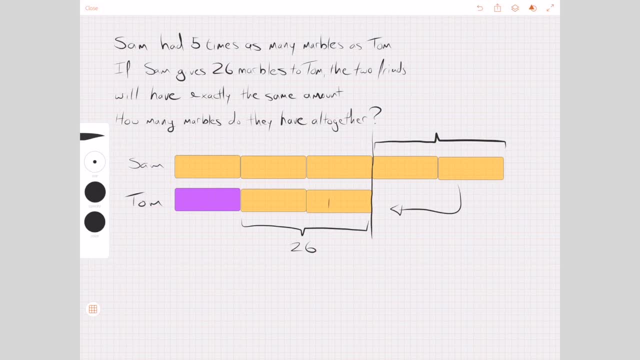 to have the same amount of marbles, that they're going to have the same amount of marbles. So, if they know that two of these rectangles equals 26,, then one of these rectangles must equal how much? 13,, because each one of these bars, of course, is, uh, the same size as 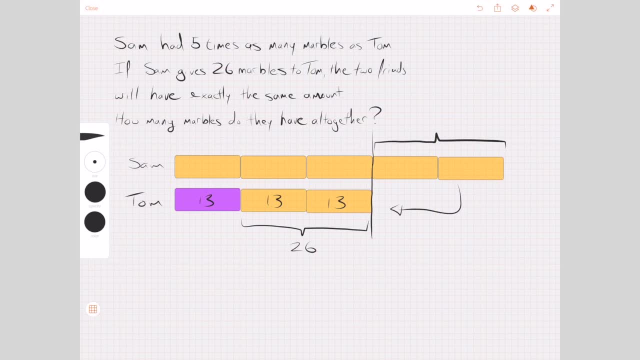 the other. So if these two are 13,, then all the bars have a value of 13.. And to look at our question now: how many marbles do they have altogether? You can see that the problem is quite straightforward to solve here. It's a very basic calculation: 13 times six will. 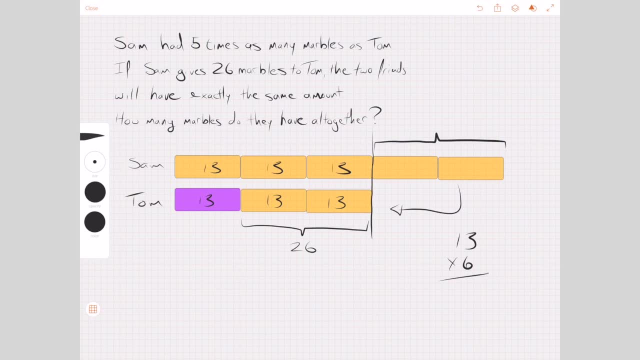 give us the answer. Um, hopefully, at this stage, children will not have to do it in the long multiplication, uh, but we'll be able to do this in their heads, uh, and may even write it this way, Right, Okay, I hope that's helpful. Um, now the other thing I want to, just very quickly. 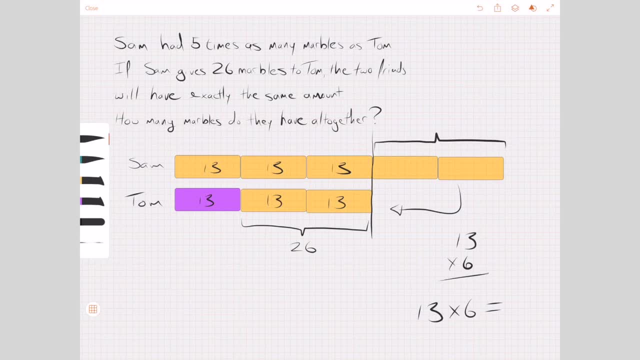 talk about is what happens when children are struggling with these types of word problems. Well, what I hope you notice is that the mathematics here, in this case this calculation over here, is fairly straightforward, and that's done on purpose. We want to see children- I mean, if my children have problems with these types of problems, 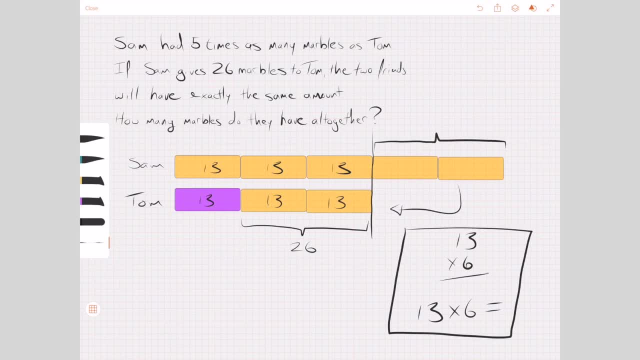 let's say, if I have a child that's struggling with this, you know this is a kid that's struggling with this. So I want to see children with really tedious computation at this stage. We want them to read the problem and try to make sense of it. Some children will naturally struggle. 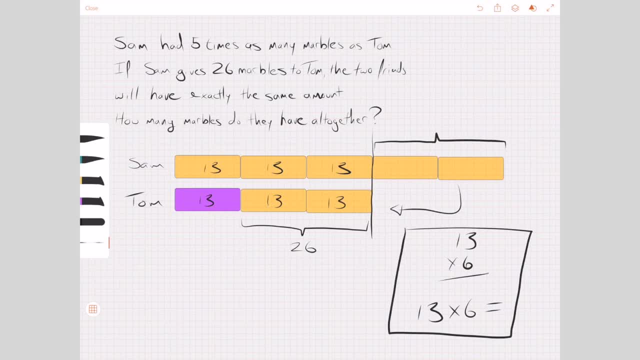 with this. So what are some of the things that you might be able to do to help children? Well, often, when children struggle with problems like this, the types of things that they'll struggle with is the amount of details that they have to deal with. So, in this case, here,